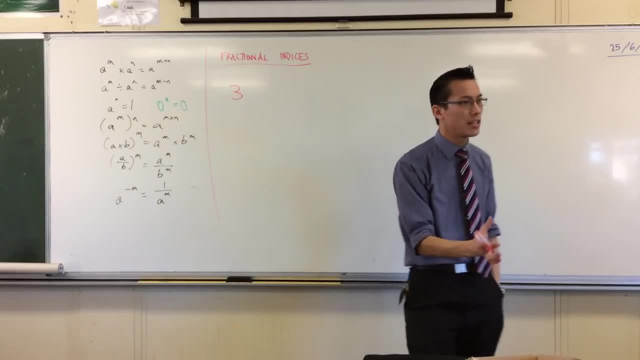 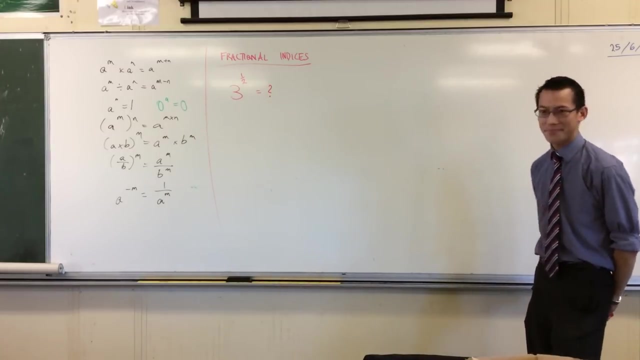 Let's think of something like, say, 3, and let's put a fraction in the power. We'll start with an easy one. Let's put a half. Now my question is: what is this thing equal to? Now? see, here's the problem. 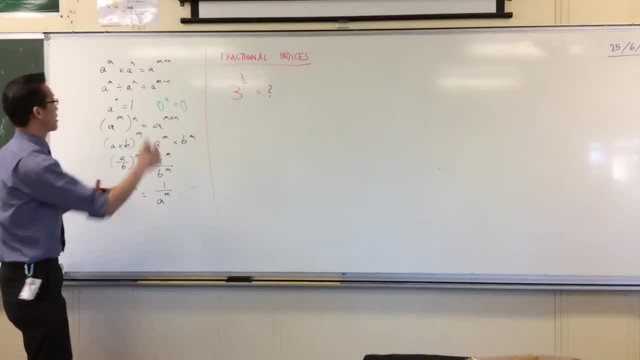 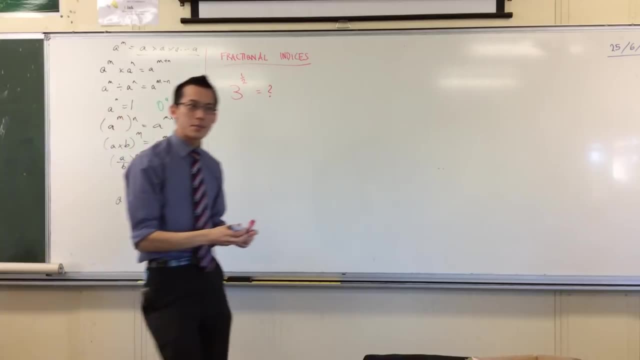 The whole idea of indices is not a law, but it's like a to the power of m means you multiply the number by itself And you do it m times, right, But I don't have a number of times Like: what is it? 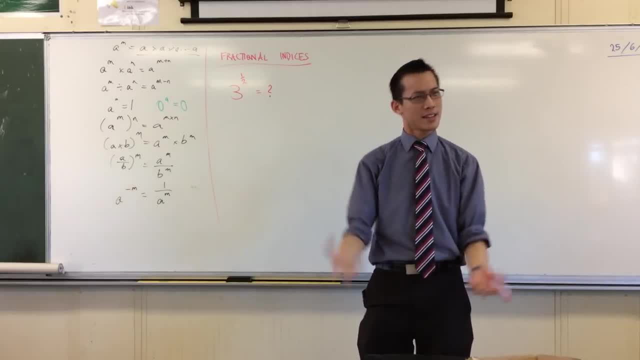 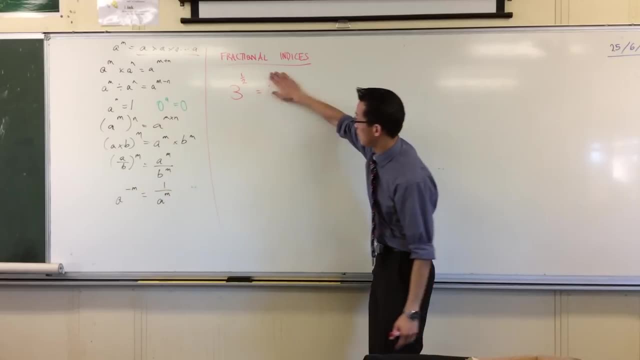 What does it mean to multiply a number by itself half a time Like that doesn't really make sense. okay, So here's the way I'm going to approach it. I'm going to think about these laws and see if I can do something that will make sense here. 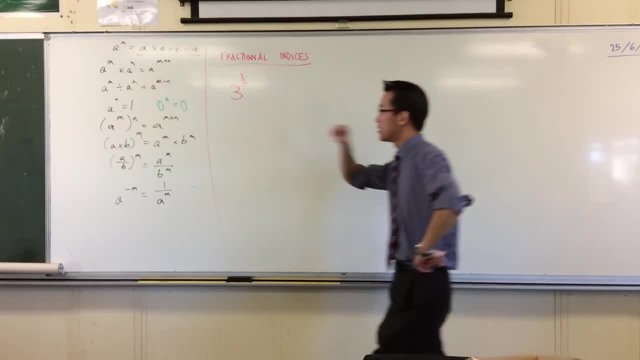 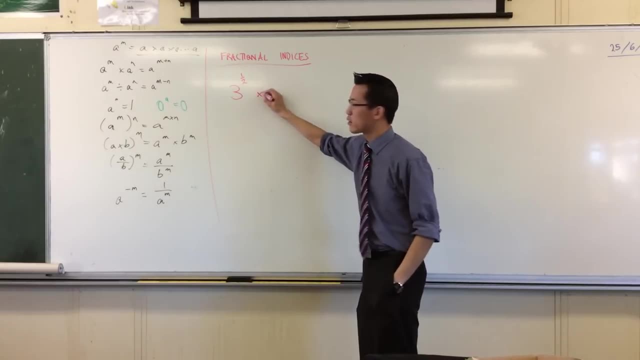 Suppose. which way shall I take it? Let's go this one, Yeah, this one here. First one, the very first one, the simplest one. If I were to multiply this number by another number- same base- for the purpose of illustration, I'm going to make the power the same as well. 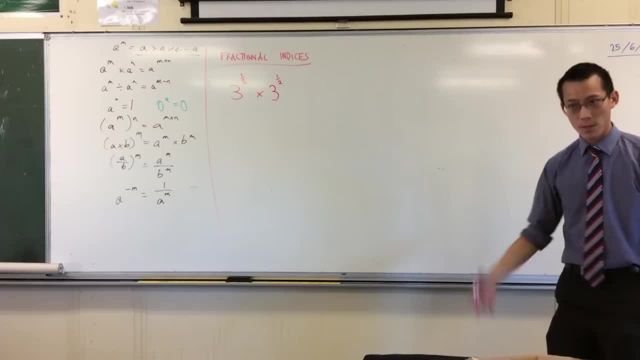 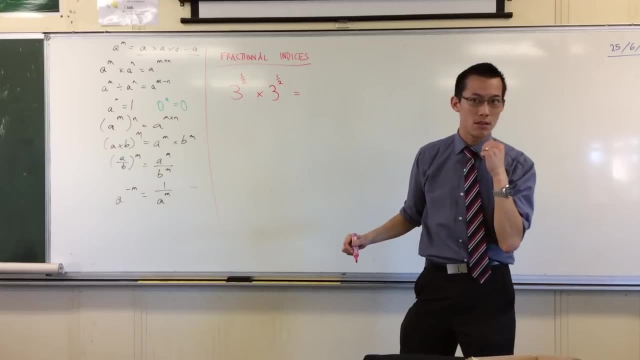 Okay, Three to the power of a half, times three to the power of a half, According to this first law that we established ages ago. what should I do to the indices? I should add them Like: so: Well, what's a half plus a half? 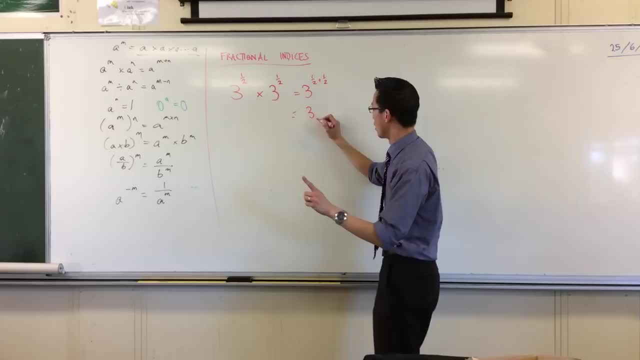 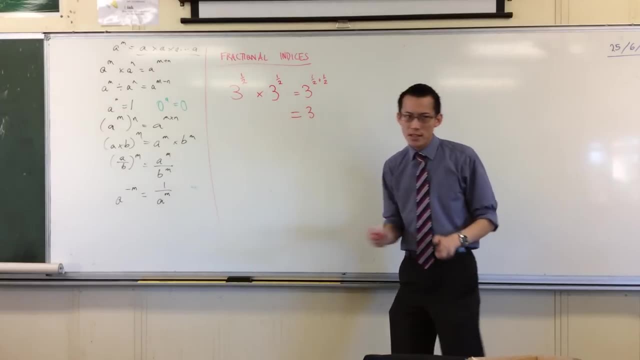 It's just one right. Hold on Three to the power of one is just three, Like that, Hold on a second. What does this mean? We're trying to work out what is three to the power of one, Three to the power of a half. 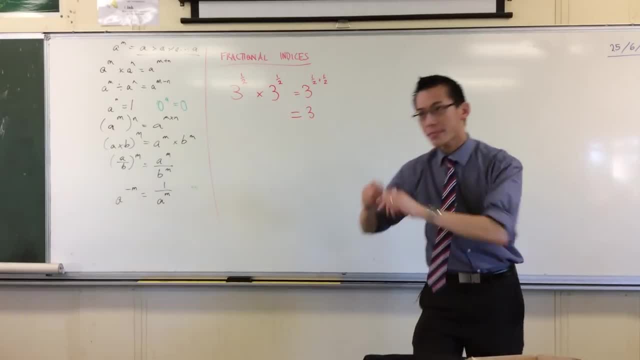 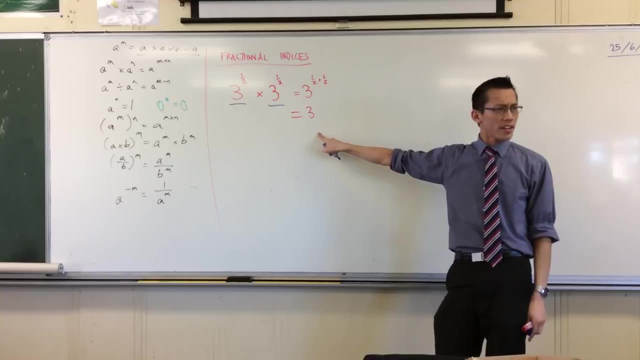 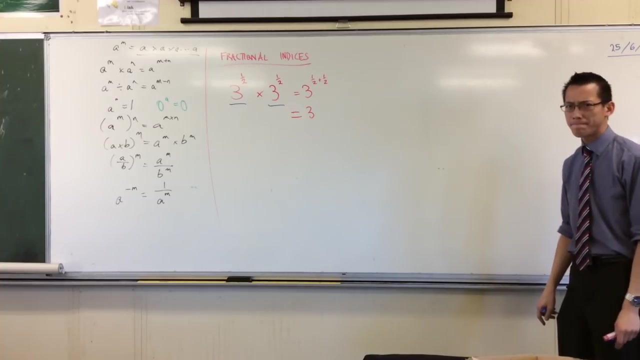 What is that thing? Now, what we've noticed is that this: if you multiply it by itself, you get three. What number do you multiply by itself to give you three? Now, we need some new notation here. You actually all know this number. 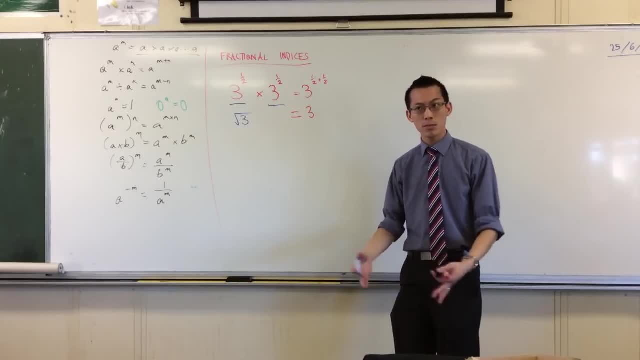 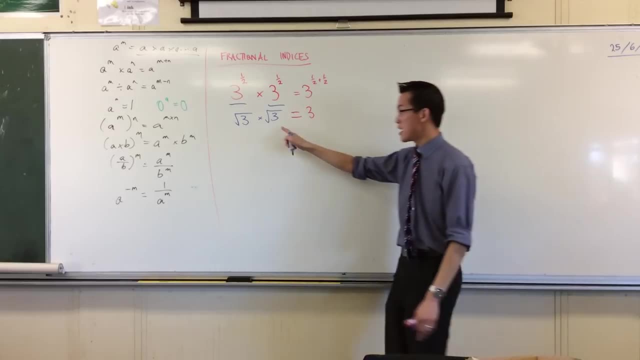 We call it the square root of three. If you multiply the square root of three by the square root of three, you get three. In fact. that's what square root means. It's the number that you multiply by itself, and it will give you back this guy. 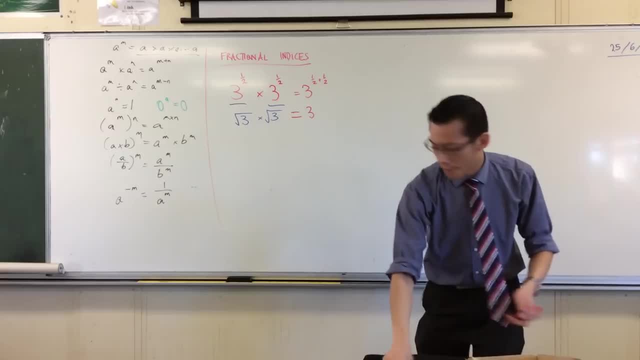 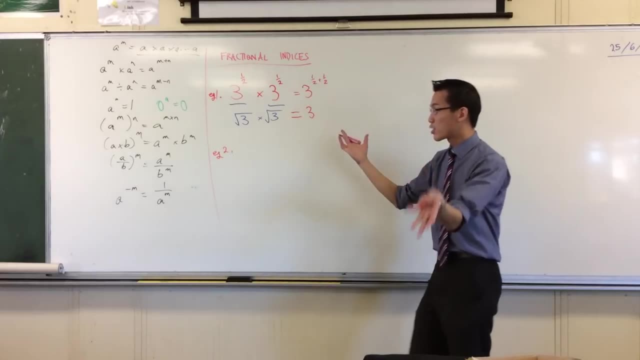 Let's push forward. Let's have a look at some other fractions. Let's try, for instance: so this is example one. Let's do example two. Let's go with a number like, say five. Let's take a different fraction up there. 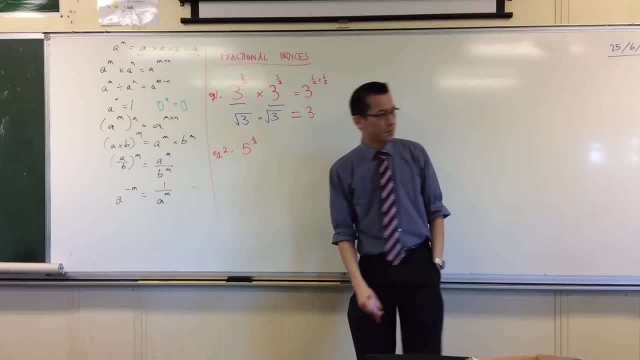 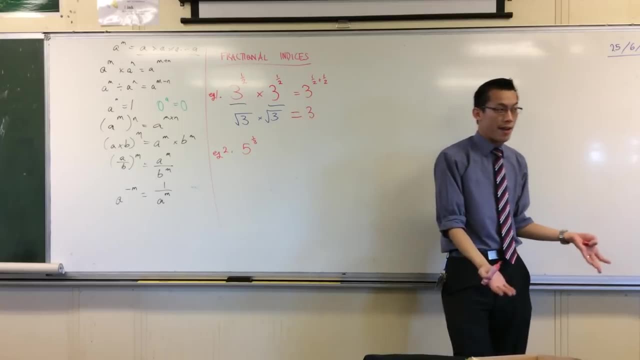 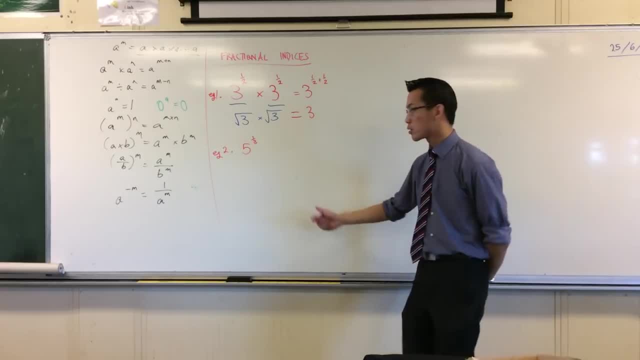 whatever that is, what's it equal to? I'm going to multiply it by something. Any suggestions? What should I multiply it by Seven? I can multiply it by seven, but would you get much meaningful out of that? Would you just multiply it by the second? 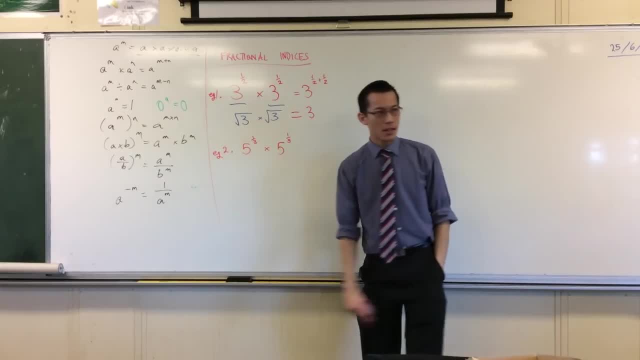 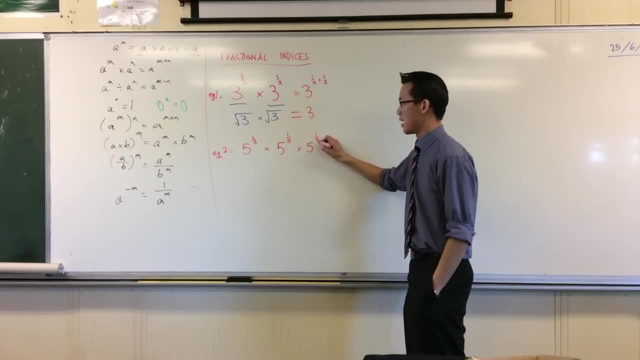 I might multiply it by itself. For reasons that will become clear in a second, I'm going to multiply it by itself one more time, Three times rather than two. I wonder if you can see where I'm going. The denominator is three. 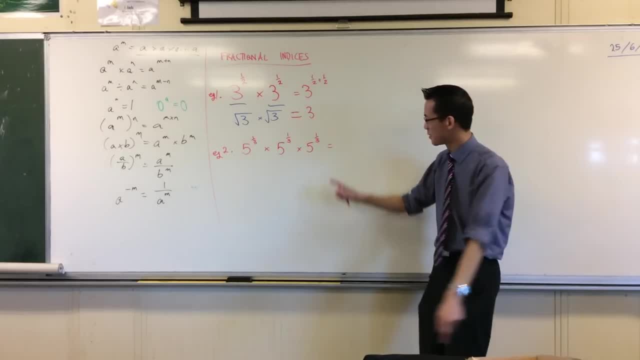 Hold on, Be careful about your numbers. right, It is about the denominator Multiply numbers, all with the same base. So what do I do with the indices? Add them. I'm going to add them. So I've got a third plus a third plus a third again. 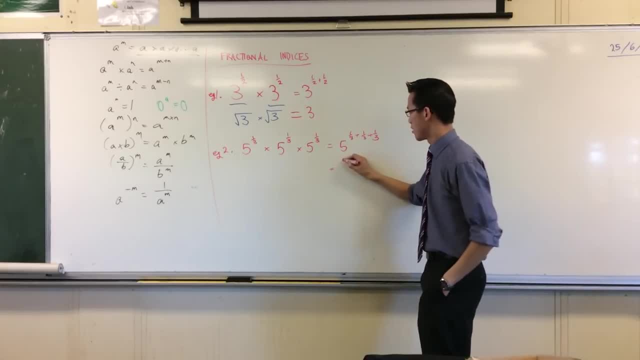 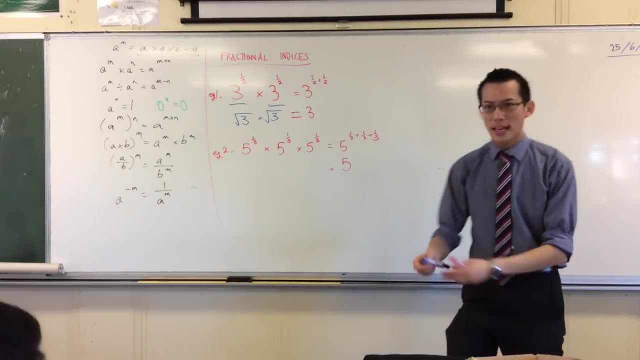 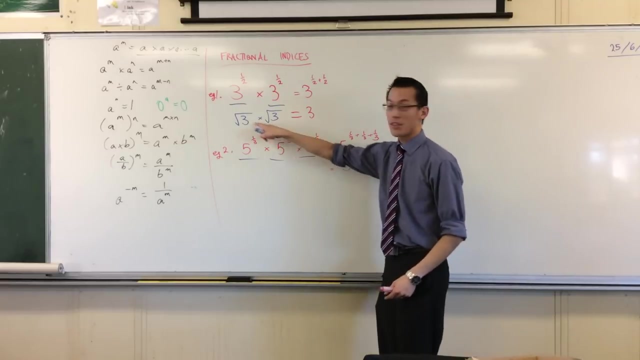 That's one, isn't it? Third plus a third plus a third, The power of one is five. So I've got some number, And when I multiply it by itself three times, I end up with five. Well, here we call this the square root. 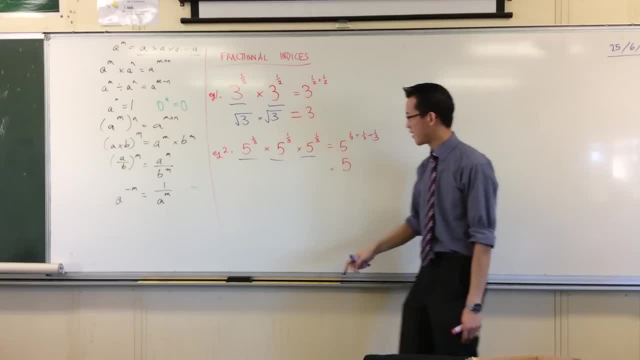 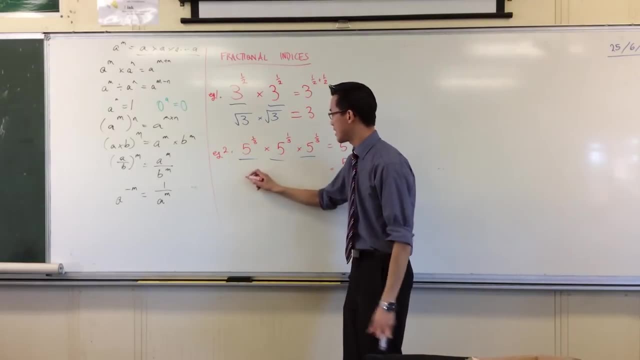 If you square three- the square root of three- you'll get the three. We call this a different number. It's not the square root, is it? It's called the cube root. We write it like this in a very similar way. 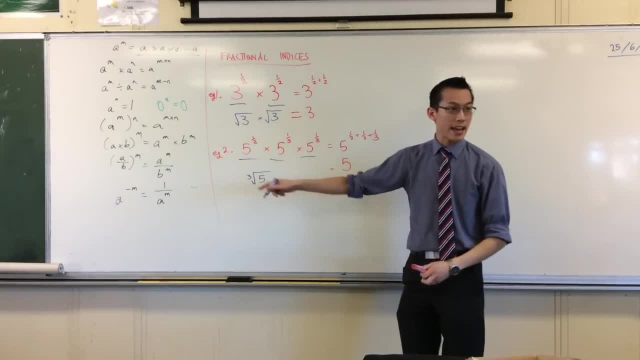 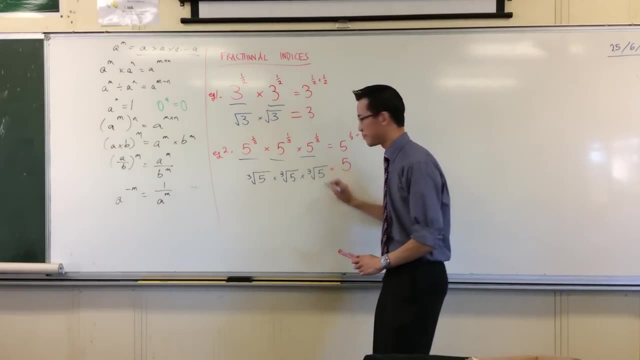 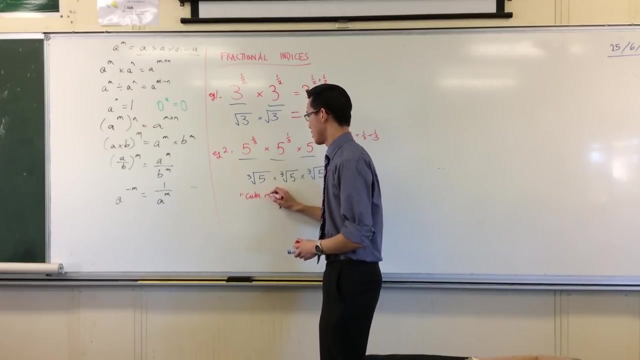 We write it with a three. outside there I read that as the cube root of five. Okay, Cube root of five. In fact, I might even write that for you. Why, to the times, rather than the blocks, Where, On the cube plus the cube. 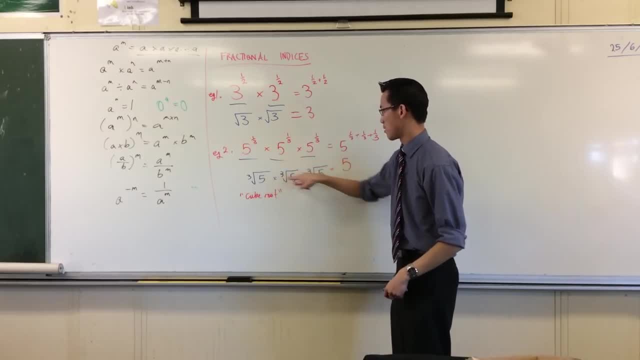 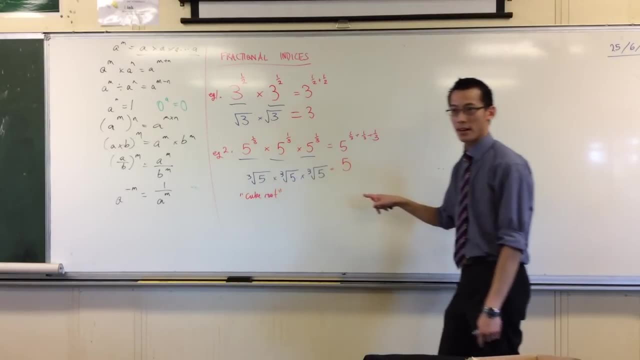 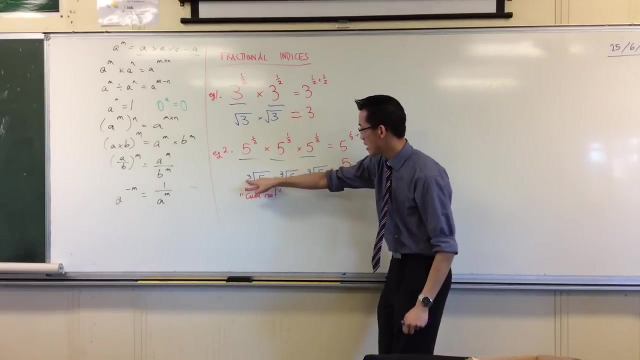 Here, here, here, Because there's multiplication there. If I added these together I wouldn't get five. I have to multiply them together to get five. Is the three there? because there's three fives. Do you mean this three or this three? 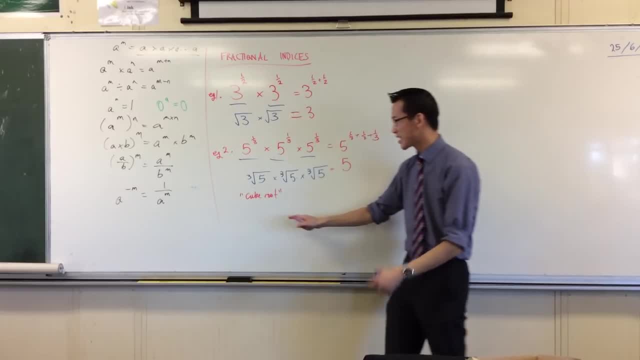 No, you have three where the square root is Yeah. okay. So that three there indicates it's not the square root. That's what it usually means, It's the cube root. And I can actually keep going. I could not just have the square root or the cube root. 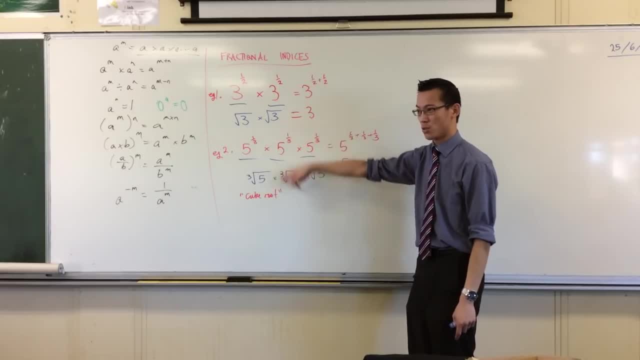 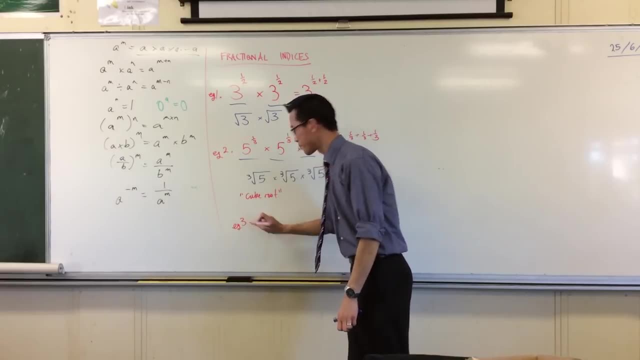 I have different other kinds of well, not twos or threes, but let's do some other crazy number, Let's do ten. Here's my third example This time I'm going to go to. let's try this law instead. 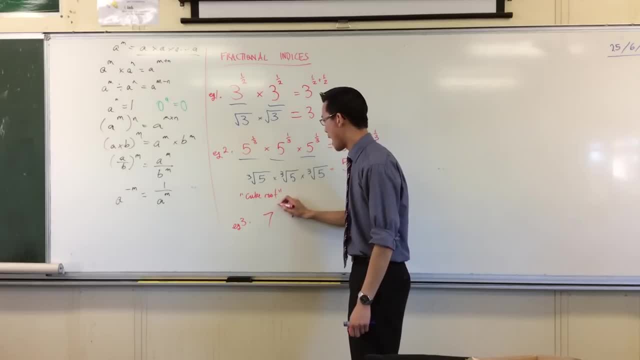 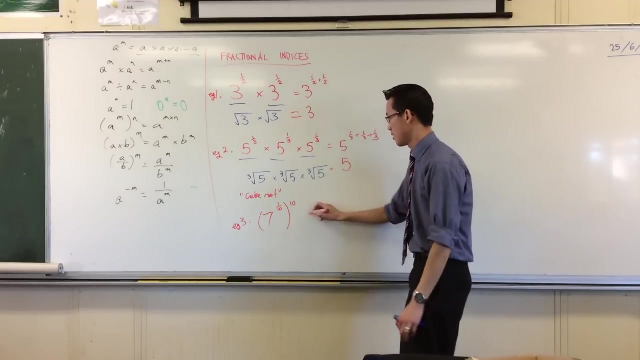 because I don't want to write this out ten times. Let's go seven to the power of one tenth. Now if I multiply this number by itself ten times, See that That's multiply whatever's in there by itself ten times. According to this law in here, one, two, three, four. 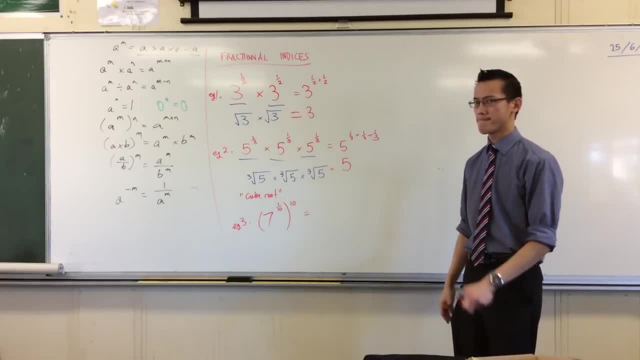 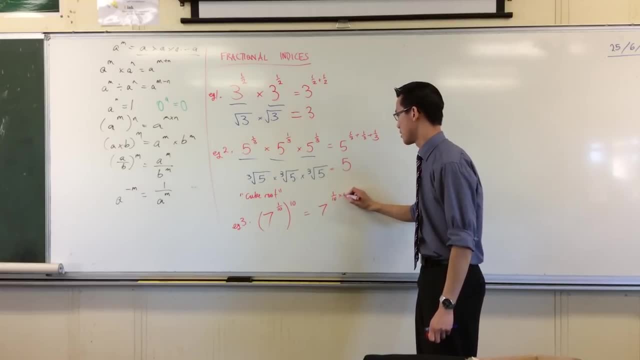 this is power over power. So what do I do to the indices? I multiply them, right, You see what's going on. So that's a tenth times ten, That's just seven to the power of one, which is seven. So what's going on here? 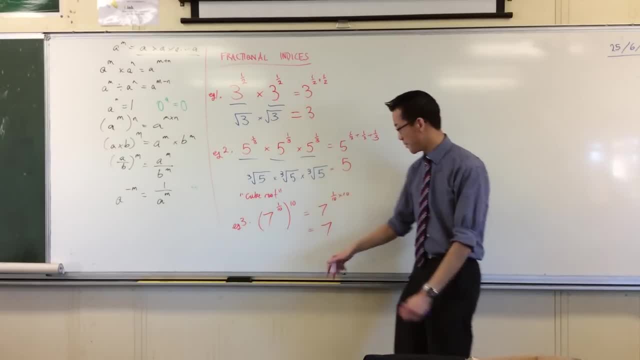 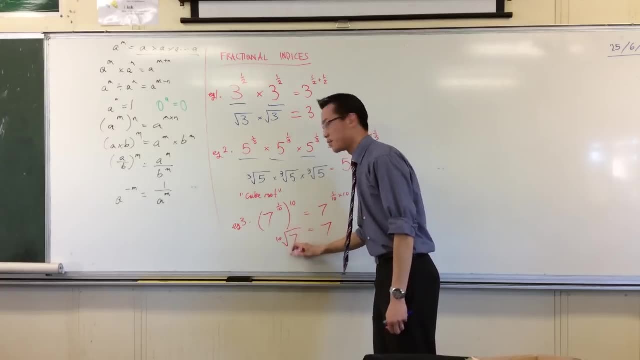 This number is the number that you multiply by itself ten times to give you seven. I would call that, rather than the square root or the cube root, I would call it the. well, I just call it the ten, Because the numbers are going to keep going. 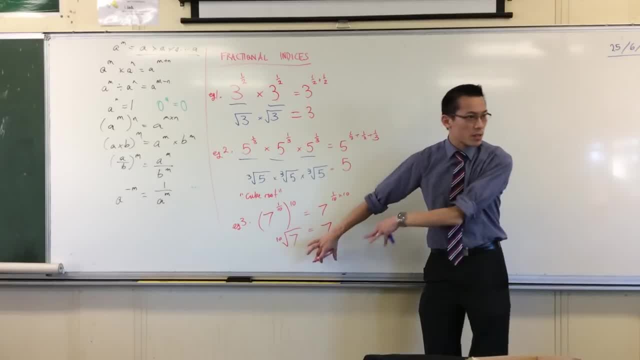 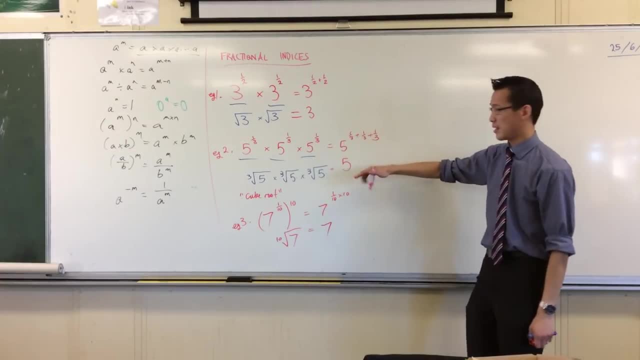 eleven through twelve, through whatever. That's what's going on. That's a really big example. You don't really need to worry about that, But I'm just showing you. you can. These are the main important ones that we're going to see here. 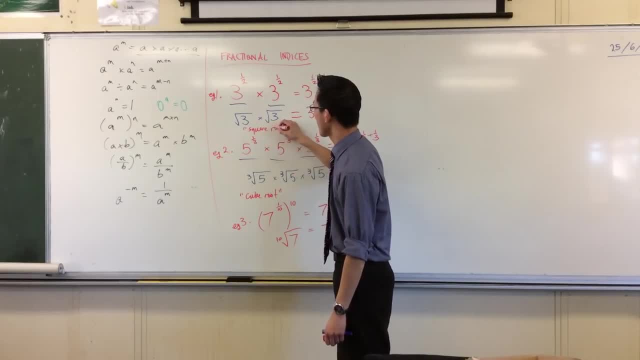 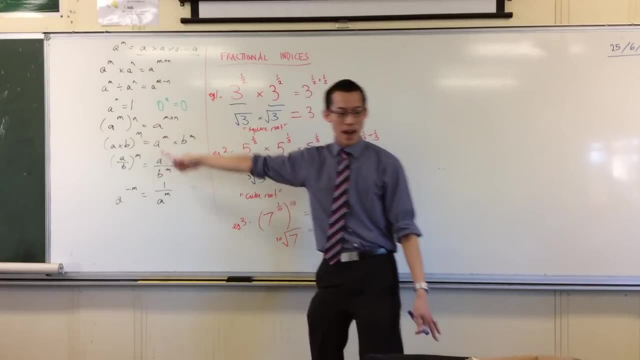 I wonder if that's the wind taking out a power station. So you've got the square root there and the cube root there. So let's bring this back to our list of laws, which, again, it's not just. why are these true? 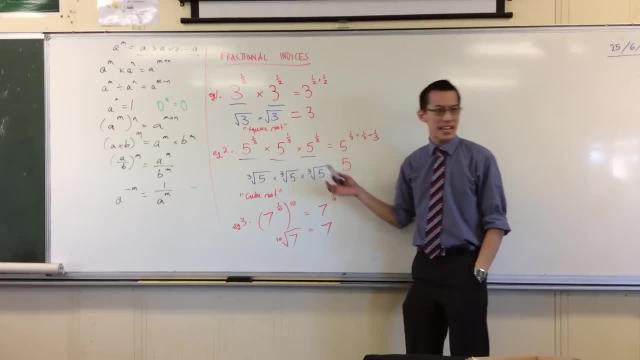 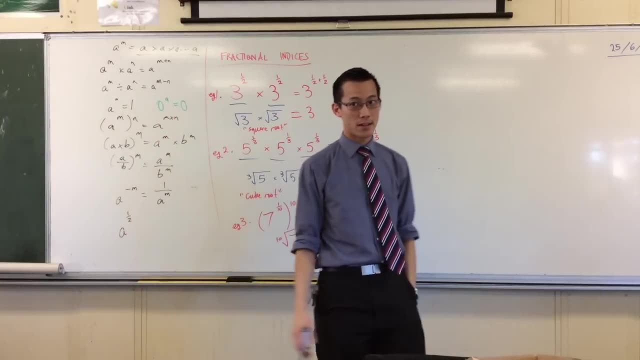 Just because we said so. They're true, because you can see. that's how the rules of the game work. So I'm going to write in these two A to the power of a half. When you see that What that really means is: 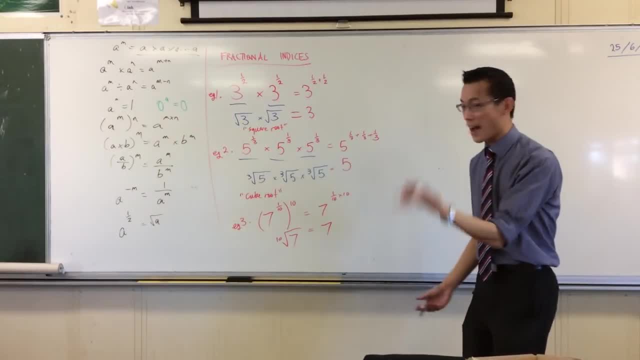 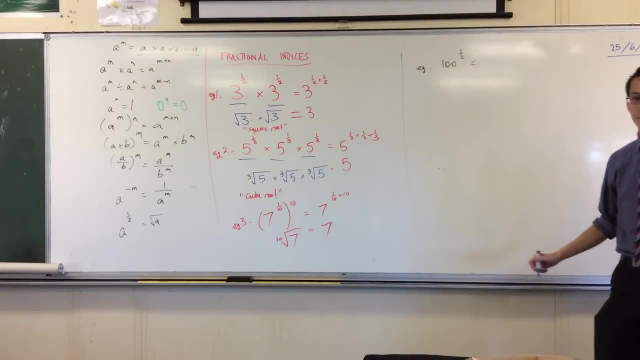 the square root of A. So if I gave you as an example, a hundred to the power of a half, A hundred to the power of a half, That's the square root of a hundred, Which is the square root of a hundred. 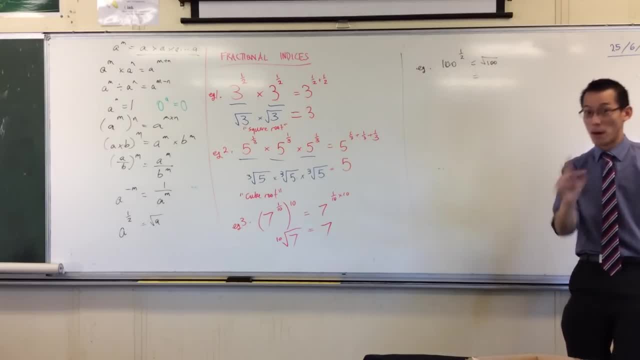 What's the number that you multiply by itself to give you a hundred. Multiply, Multiply, It's ten, And your calculator can do these too. It can do the square root In exactly the same way. this is kind of like the same law, but with another number. 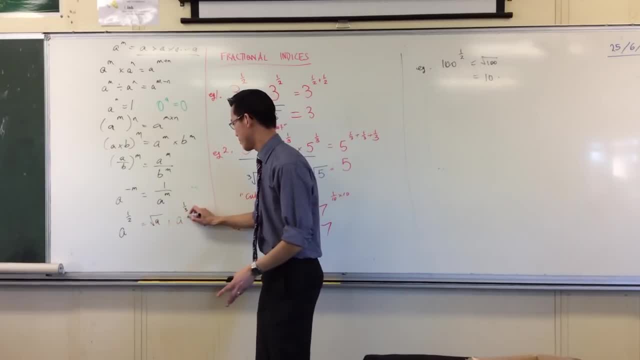 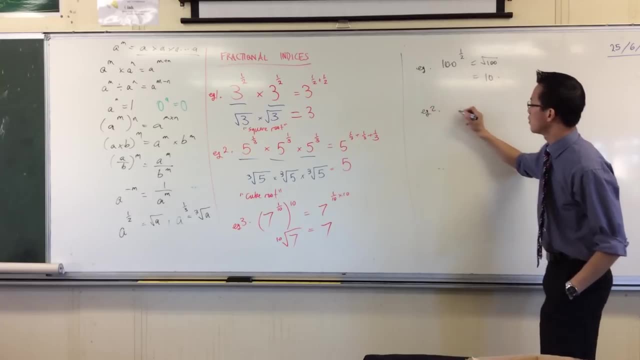 If you see, A to the power of a third, it's not the square root, it's the cube root. So, for instance, one of the key numbers I know, if I gave you this example, 64 to the power of a third. 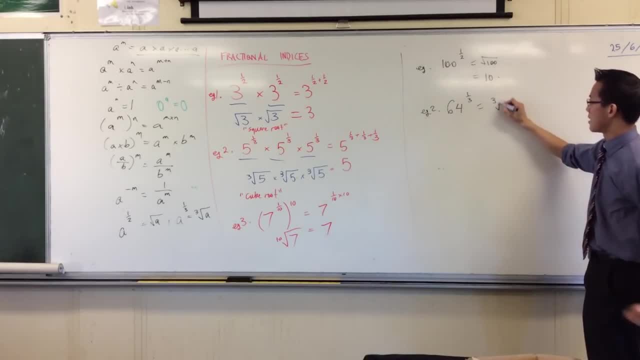 Now, you might not know this number off the top of your head, and that's okay, But it's the cube root of 64. There's a number. If you multiply it by itself three times, you'll get 64.. Does anyone know what it is? 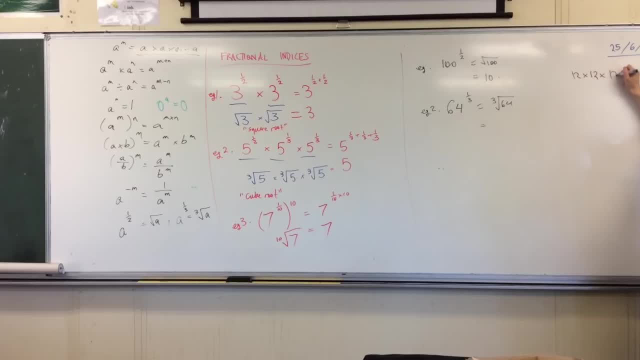 Twelve, Twelve times 12 times 12.. That's going to be 144 times 12.. Which I think is going to be- oh man, I shouldn't have done this- 1140 plus 288.. It's 1728.. 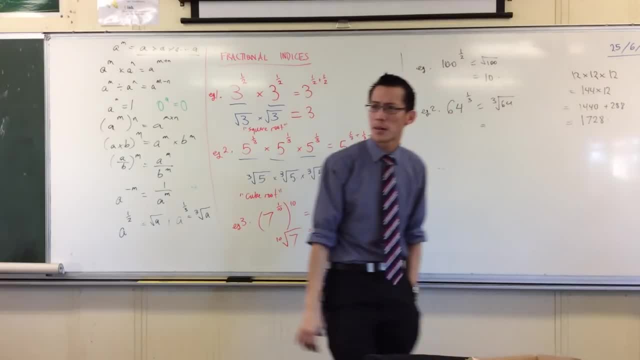 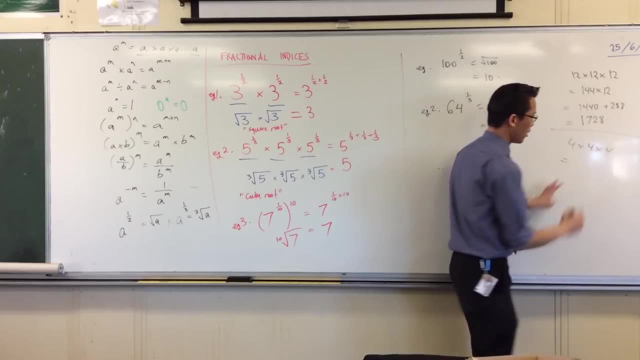 That's not 64. It's way too big. It must be something much smaller. Yeah, Four, Four, Let's try four. Four times four times four, You do the first pair. What's four times four Sixteen? 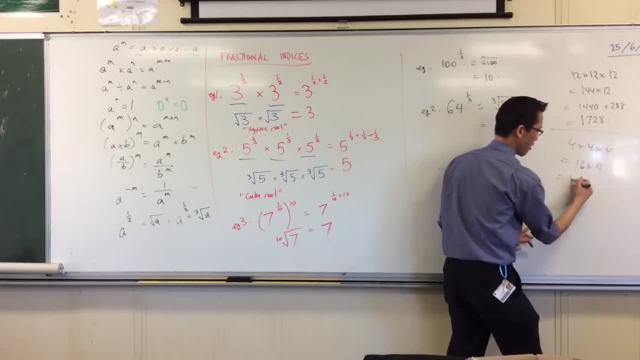 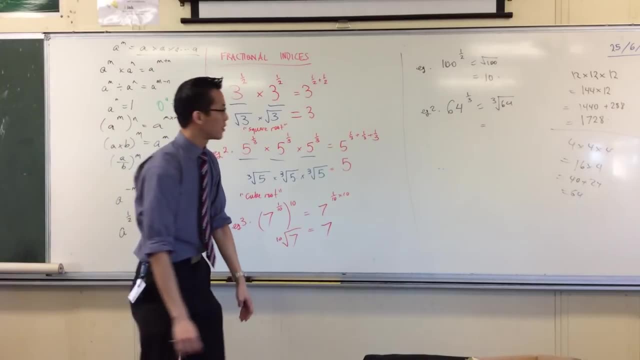 Sixteen times four. If you do those, that's 40.. If you do those, it's 24.. It's 64. It works. The cube root of 64 is four. That's a less common number, but now you recognize it. 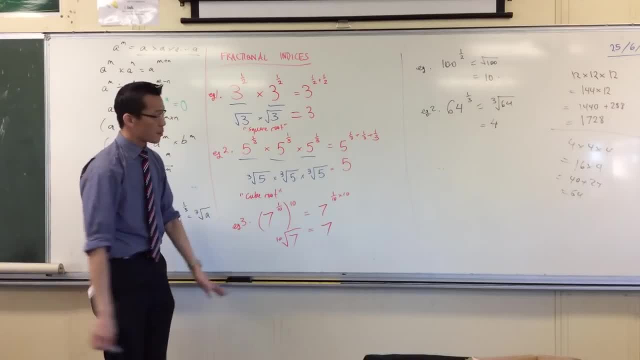 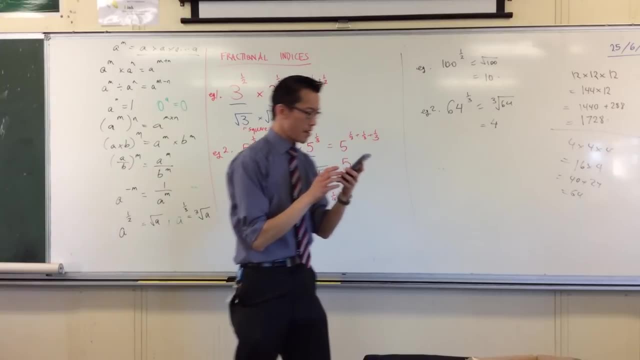 so you can use that as an example. Hold on, Let me write that down. No problem, That's okay. Whenever you're unsure, get your calculator out and you will actually see. let's see, where is it. You've got your square button. 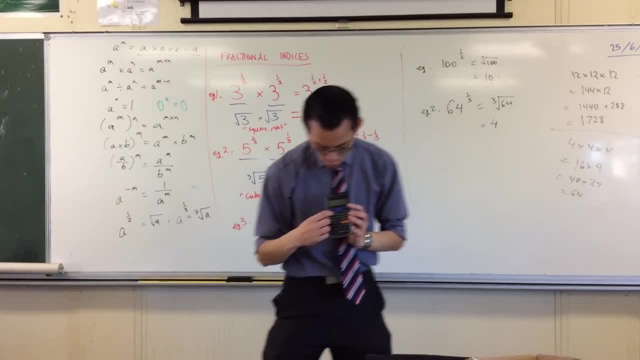 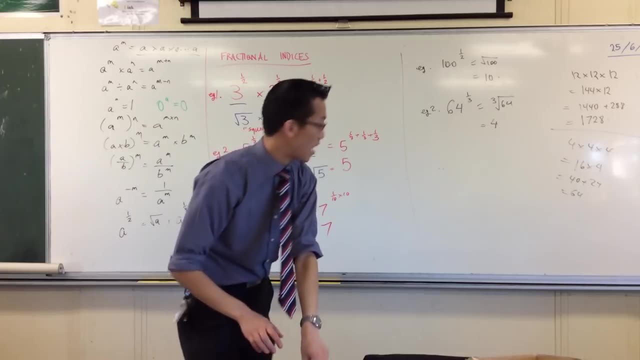 and right next to it is the square root, so they're beside each other. You've got the cube button, and just below that is the cube root button, so you can use that as well. For instance: let's see, Let's do one more. 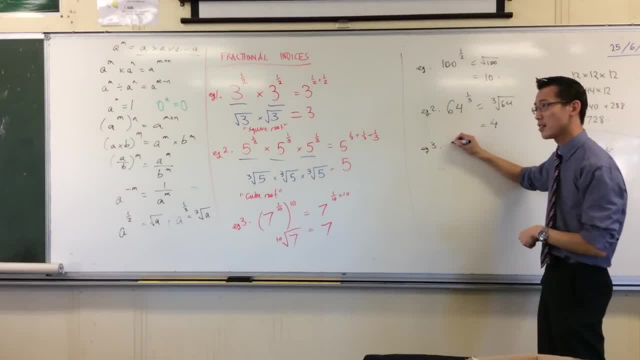 This is going to be well, let's try this. I think it's 125.. Now, what's the cube root of 125? Dunno, You get your calculator out and on mine it looks like it's right above the square root button. 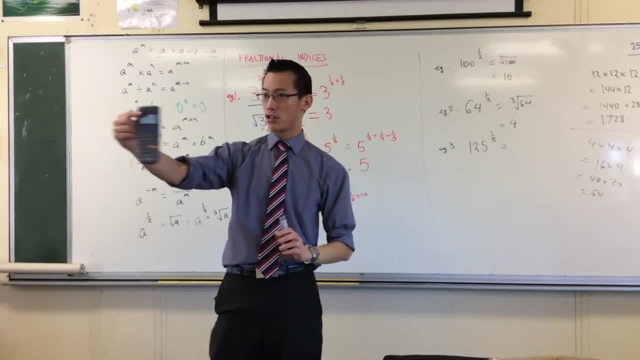 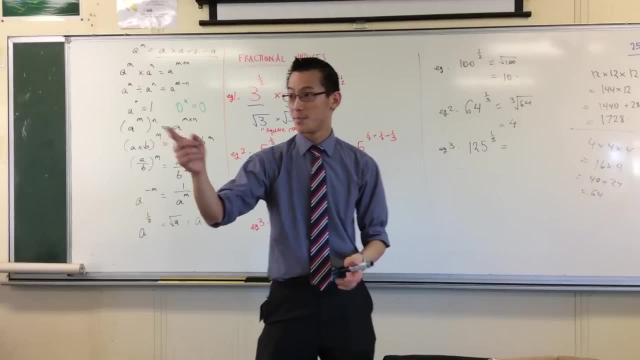 You go shift square root and you can even see that little cube root icon appears. Then you slap in your 125, and you hit equals and what do you get? Say it again: Five, Five's. exactly right Now, by the way. 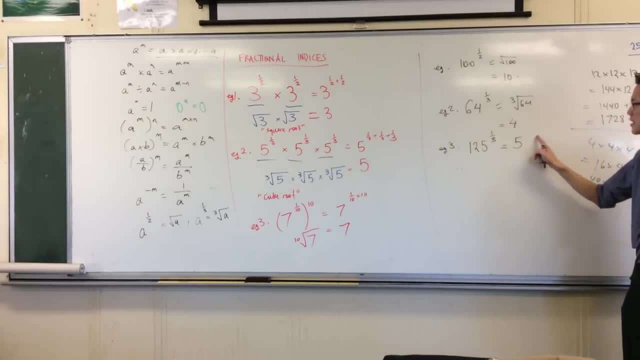 you can test this out. If it's the cube root, that means if I multiply it by itself three times, I should go back to the original number, 125.. Five times five times five, That's 25 times five. Sure enough, that's 125,. 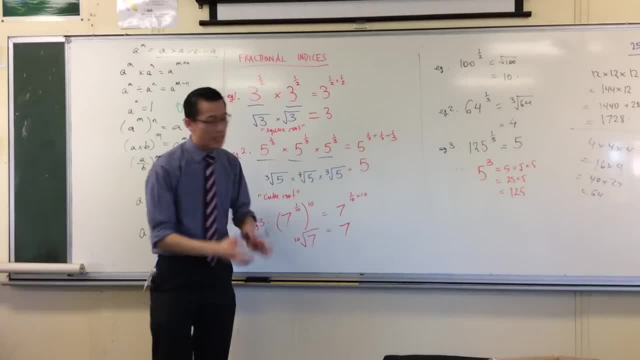 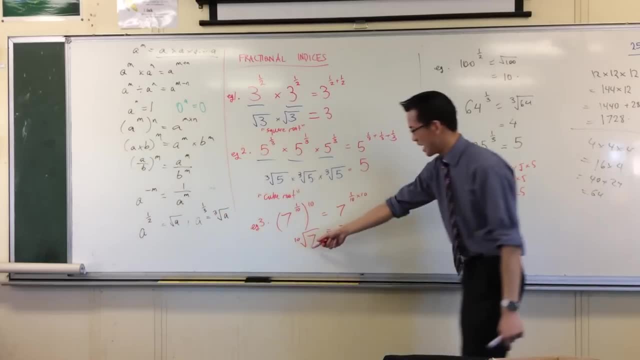 and you can check it out, okay. So, in summary, you have these fractions in the index. You're going to get square roots or cube roots or tenth roots or some number like that. okay, The most important ones that you'll see.